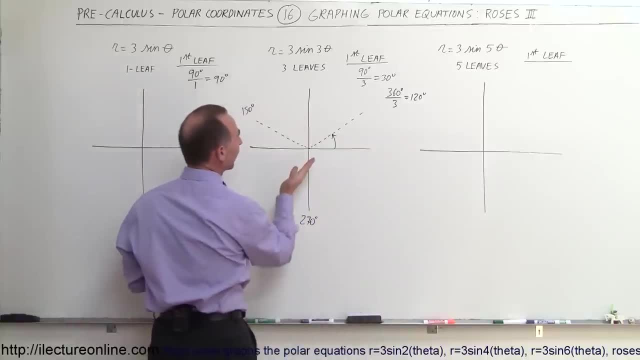 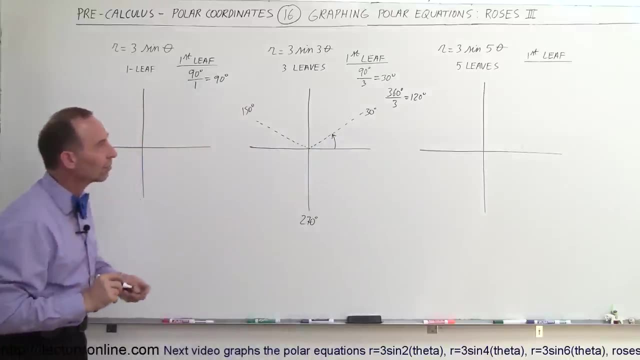 locations where the three leaves are found. so at 30, at 150 and at 270. let me put 30 degrees down right there. so that's how we find the location of the leaf In the five leaf rows. the first leaf is going to be found by taking 90 degrees. 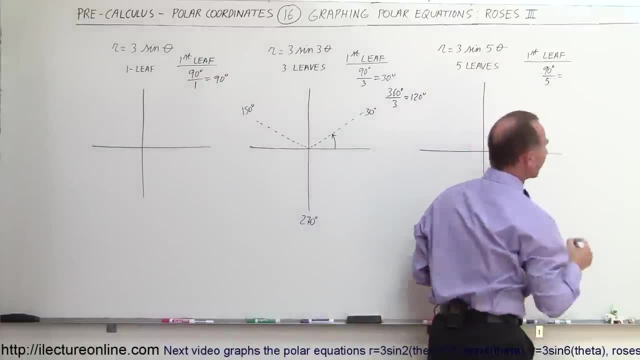 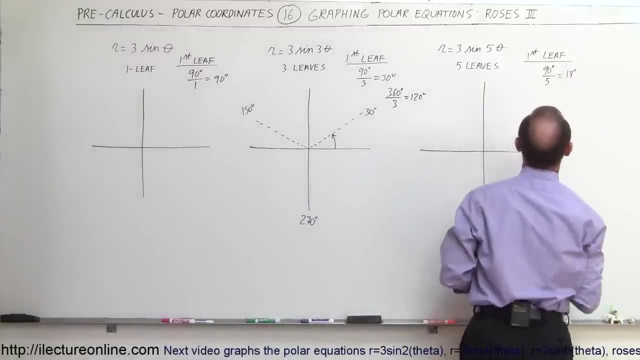 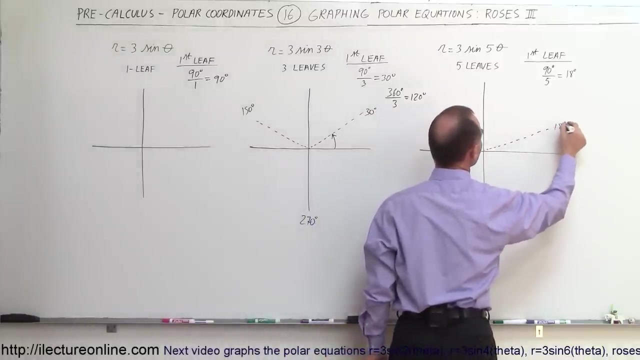 divided by the number from the angle, which is 5. so 5 goes into 90. that would be, hmm, 18. that would be 18 degrees, wouldn't it? 5 times 18 is it's a 90. so that means the first leaf would be found at an angle of 18 degrees. now, where the 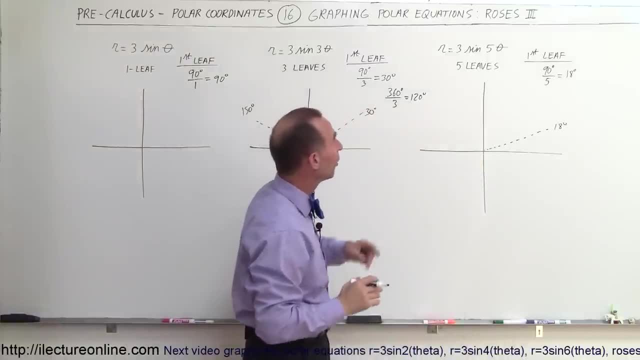 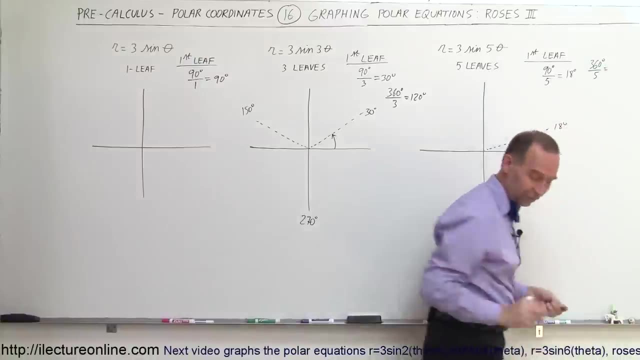 other leaves. well, there'll be five leaves. they're spaced apart in equal angles, so we take 360 degrees and then we find the first leaf, which is 90 degrees divided by 5, and what do we get? 5 times 360. I better make sure I get this right. 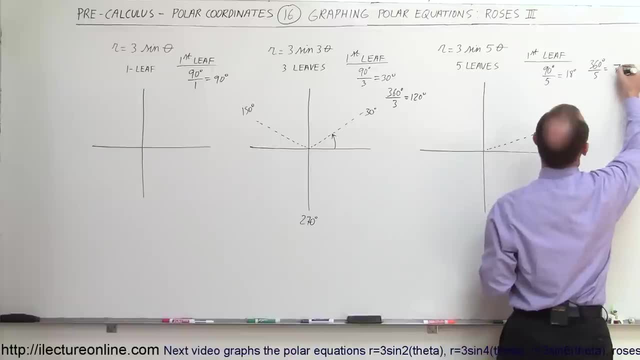 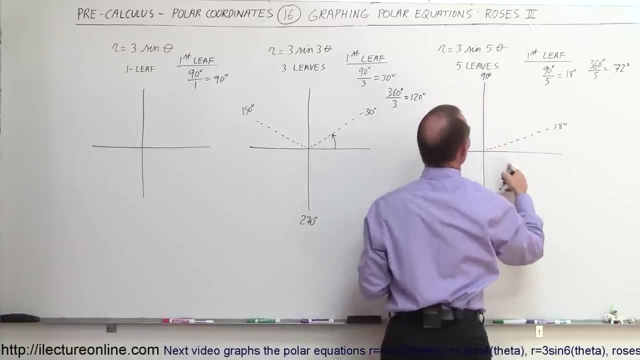 divided by 5 equals 72 degrees. that's right. so every 72 degrees. so add 72 to 19, that gives you 90 degrees. so there'll be a second leaf at 90 degrees. a third leaf would be 90 plus 72, that's 162 degrees. that's would be right about. 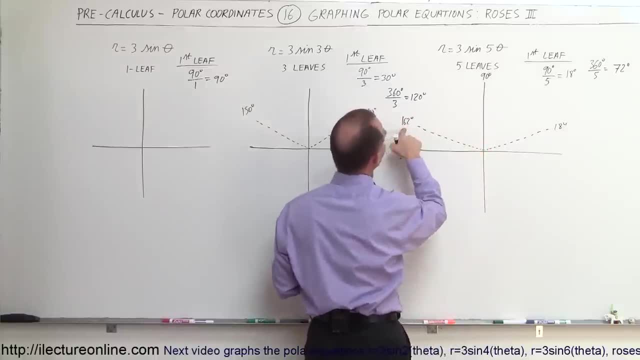 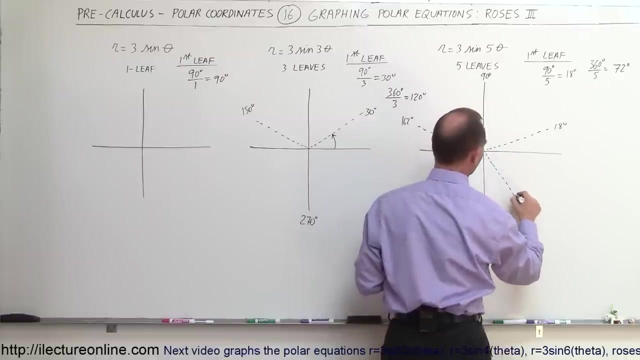 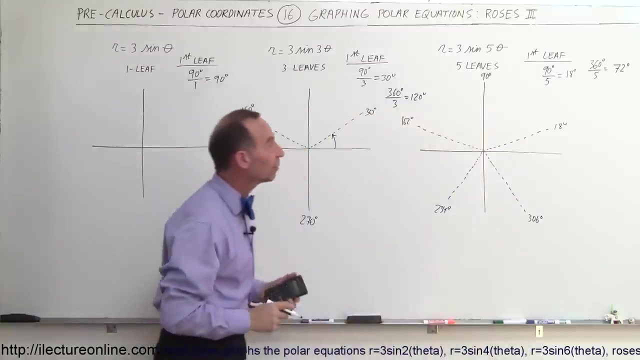 there 162 degrees. add 72 to that, that would be 234 degrees. 234, that would put us right about here. and add 72 to that, that would be 306 degrees- that would be right about here. and so we have one, two, three, four and five leaves all evenly spaced 72 degrees away from each other, starting at 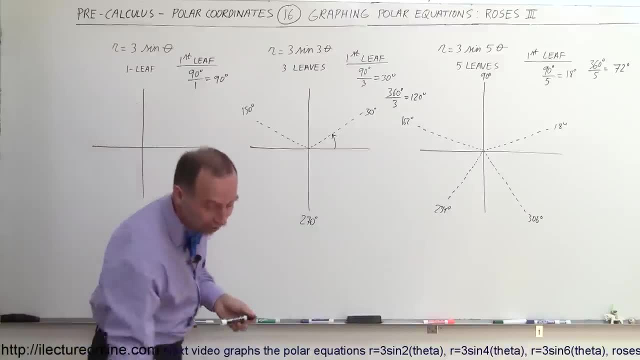 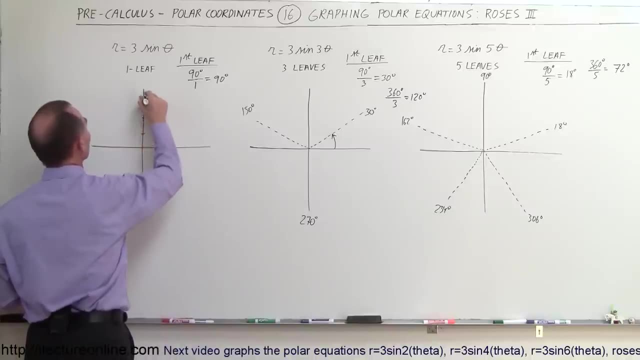 18 degrees. so that's how you determine how to graph these. now the rest would be relatively simple, with a one leaf, rows starting at the top right here, so one, two, three units away, because we have three right there. so this would simply look like a circle, just like that. the three leaf is a little nicer, like that. 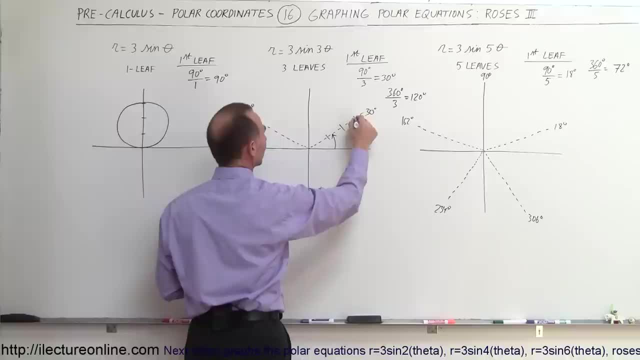 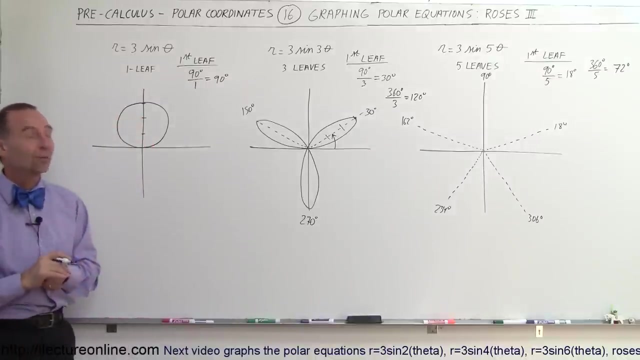 so we start at the first one over here. so one, two, three start right there. so we go like this, go like this, let me draw like this. and we come back around like this and there's your three leaf rows, for the r equals three sine of 3, theta, of course, again the number three in front.